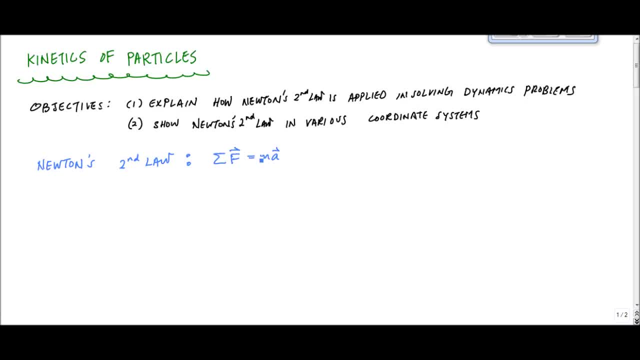 forces here is equal to mass times, acceleration. and when I see this equation I really want to try to visualize a drawing. and here there are really two really important drawings. the first, this first drawing here, is the. you know, I have this particle here. it's got all these forces acting on it, like f1, we'll say f2, and this particle could be anything right, it could be a car, it could be a ball in the air, it could be. you know, you just use your imagination of whatever you want. 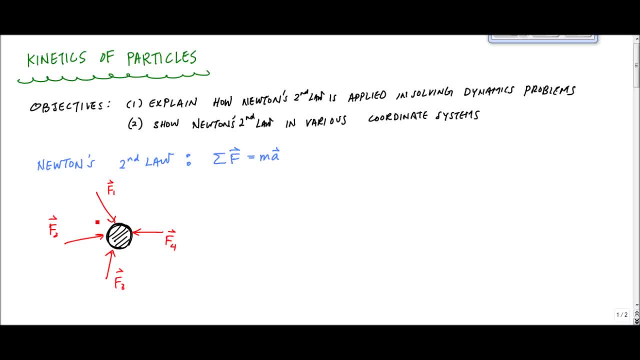 to be a particle right, and here this has all these forces acting on it. this I might call, this, I would call an external force diagram, external force diagram, and this is what you've called, maybe from statics or somewhere else, your, your, your free body diagram. so this external force diagram, and what happens is when I apply the summation of all the forces, what I get is a resultant force acting on this particle here, which 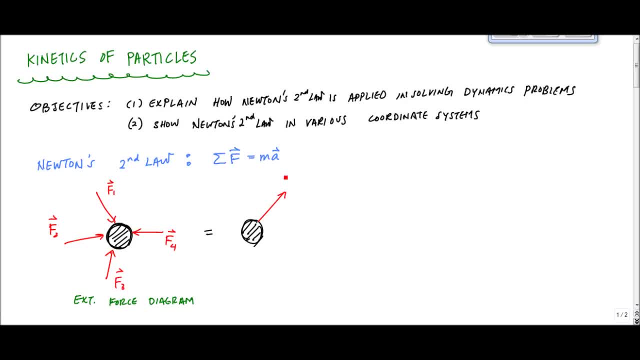 I will draw this way, like this, I'll say: there's some of all these ends up with this, right here, this resultant force, and this resultant force causes inertia or a motion here. and we'll say: here this inertia is described by mass times, acceleration. and the other drawing that's really important to make, in my opinion, is this inertial diagram. inertial diagram and being able to make 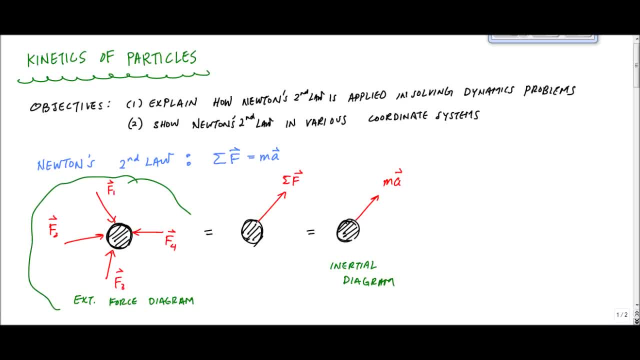 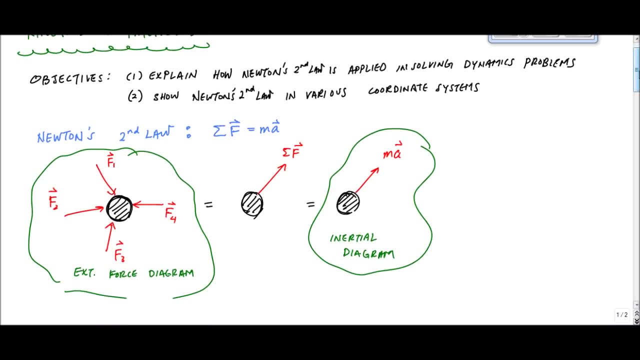 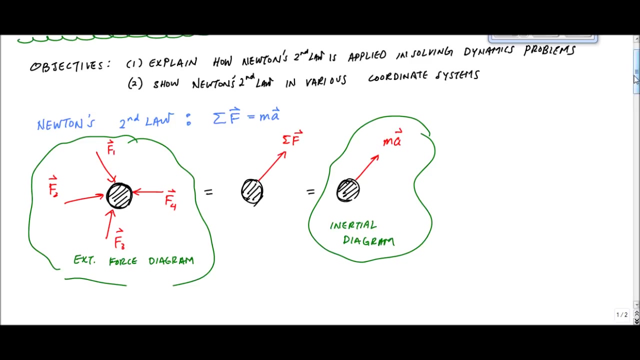 these two drawings, bam, right here, will help this drawing and this drawing here in our problems will help you to, you know, solve all your your dynamics or kinetics problems, and in dynamics or physics, whatever class you're taking here. so here you know, that's how I look at it now. the this is that that's the one thing I like to do when I apply to solve these problems. but but what's also important is now understanding, you know, how do you break these up into the 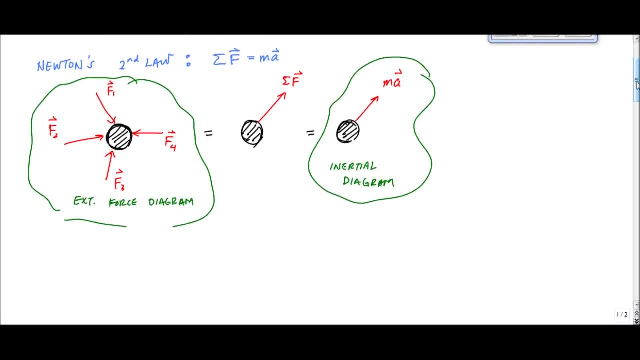 right coordinate system. and that's probably even more important in how we solve problems is is choosing the right coordinate system. you know you could be given a problem. it's a particle moving on some path, with all these forces on it and it's got some acceleration. you're asked to find the velocity or something and you have to find, and really one of the first things you have to do, besides drawing the free body diagram, is determine what kind of coordinates you're going to use and making these drawings right. and so here you have to find a program that's going to кон articles, a simple table who like to do and? and find a formula. so you're actually you're simply Ja, неп, dapat, 범, exotic, safer, Cavadares, liirs arithmetic diagram can determine what kind of coordinates you're going to use and making these drawings right. so here you're kind of thinking about how to commentate or better describe this lateralлекс, isn't it kind of like? 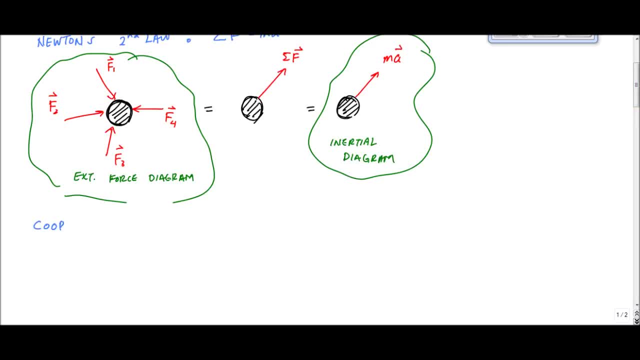 So the coordinate system that you choose is equally challenging, if you will, to solve these problems: Coordinate system right. So this is really important And the coordinate systems that you or that we have dealt with really are – there's only three kinds that we've dealt with in dynamics, or at least in engineering dynamics. 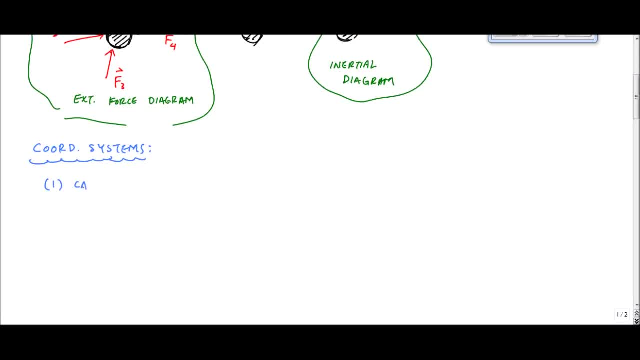 So, first course, in engineering dynamics, here you would have dealt with Cartesian or rectangular coordinate systems. So this is Cartesian or rectangular right here, Or two maybe, a normal and tangential coordinate system. This might have been called – referred to as a local coordinate system right on the particle itself. 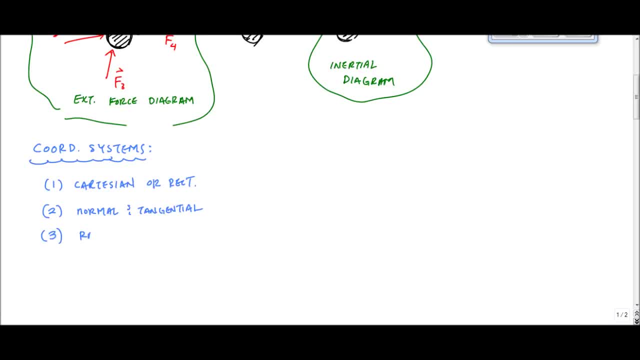 Or three, you might have dealt with a radial and transverse, And what I'd like to do is show you what all this means right here. So if I have for instance a – a particle here, let's – let's just – I'll just redraw it here. 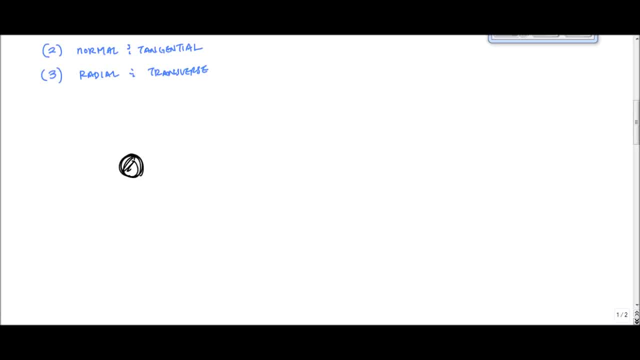 So if I have that particle here, OK, bam, my external force diagram, or whatever. I have this resultant sum of the F here And this was equal to mass times acceleration here. So I'll say, bam, mass times acceleration. Now I can choose any coordinate system to solve this problem, this basic problem here. 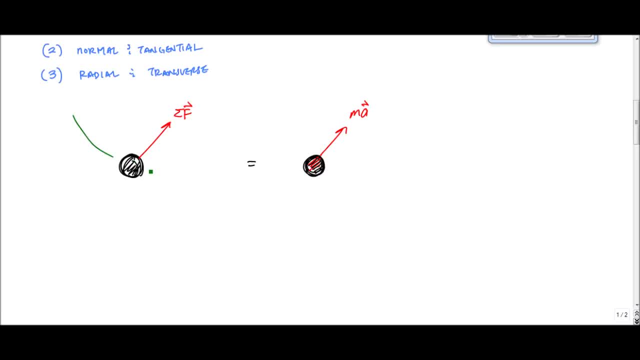 OK, One of the – and let's say, this thing is moving on a path like – like – oh, that's – ah, that'll be good enough, OK, So let's say, we'll say we're moving on this path here, like this: 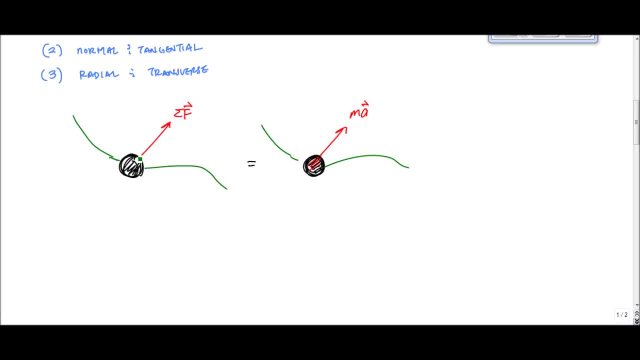 This particle is moving on this path, here that green line, And one of the first coordinate systems that you might use is a Cartesian coordinate system, or the rectangular Cartesian. Let's put that up here. We'll call that the Cartesian coordinate. We'll call that the Cartesian coordinate system. right here, OK. 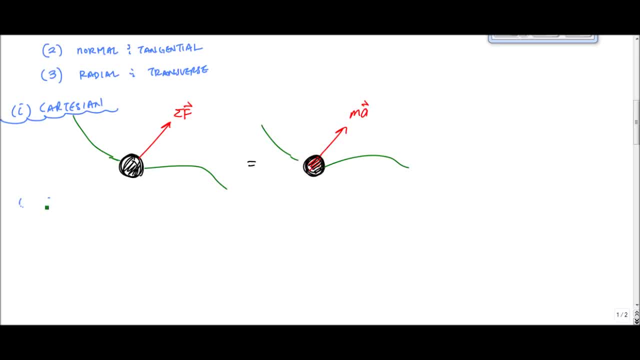 And the thing about the Cartesian or rectangular coordinate system is you need a reference, so we'll call that O some reference, And you define a plus X and a plus Y And a lot of times people do it like either right on the particle or not right here. OK, 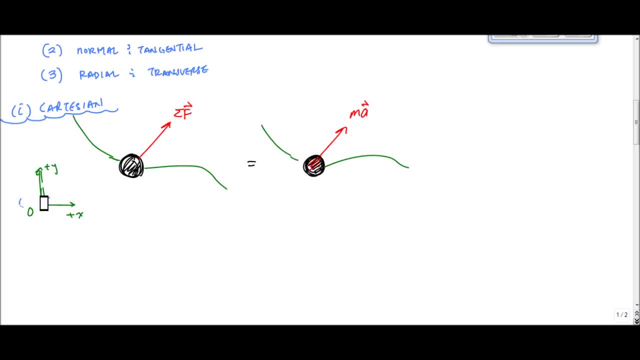 But you have a plus X and a plus Y orientation And what you do is you break up your component, the sum of the forces, into the X and the Y components. Right here, sum of the forces in the X, bam and sum of the forces in the Y. 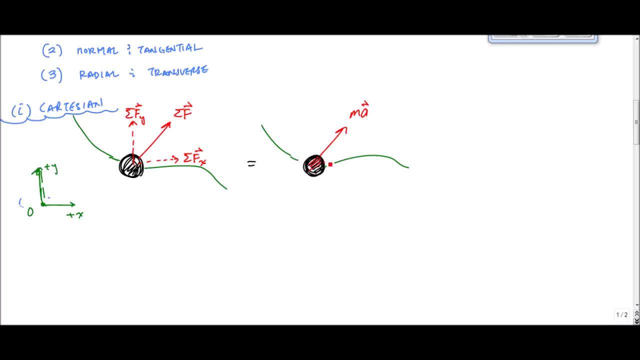 And then you would also similarly break up this acceleration vector or this inertial term right here in M-A-X and M-A-Y, right here, And you know, technically you don't even need vector symbols or anything, because you're looking one direction at a time. 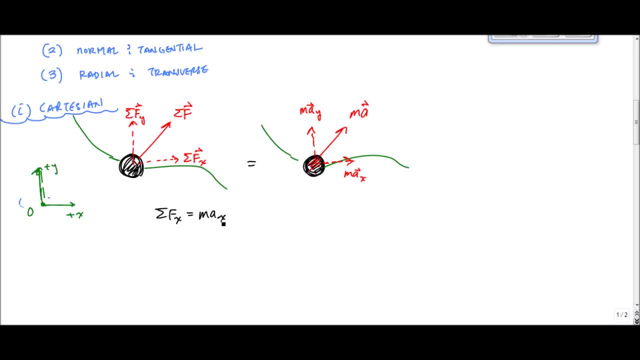 So sum of the forces in the X when you're doing this problem in 2D- OK, 2D is just M-A-X here- And then sum of the forces in the Y is M-A-Y, And this is what you know is traditional. 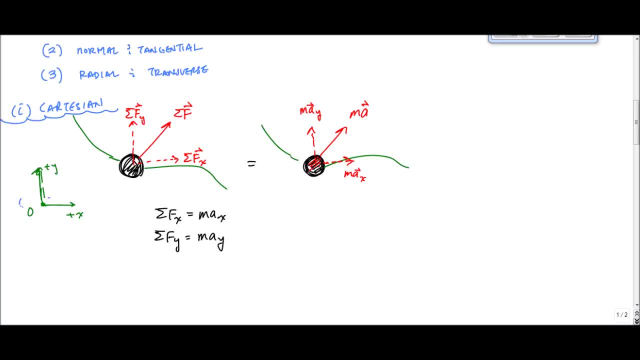 It's the easiest because you're so used to the X and Y. you follow it a lot, And this is probably a lot of places. a lot of times this is where people will go first to solve, you know, to come up with equations of motion or these F equals M-A equations. 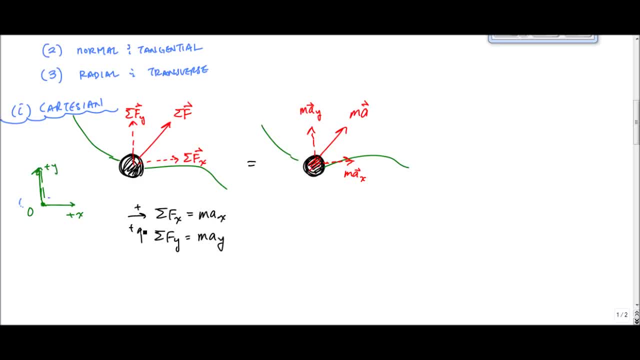 And you know, based on what you chose as the origins, these are your positive orientations right here, And this is one way you can approach the problem. Another way you can approach this problem is to choose an N-T or that normal and tangential coordinate system. if you choose N-T coordinates, 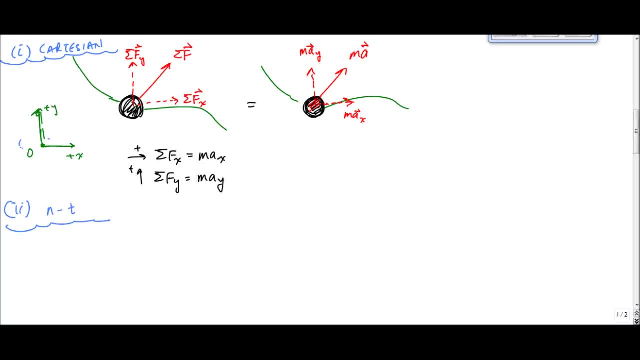 And here again, if I have the same drawing right here, so I'm going to duplicate this drawing pretty quickly. Bam, Bam, Let's go up here like this: And I have some again, that sum of the forces Bam. 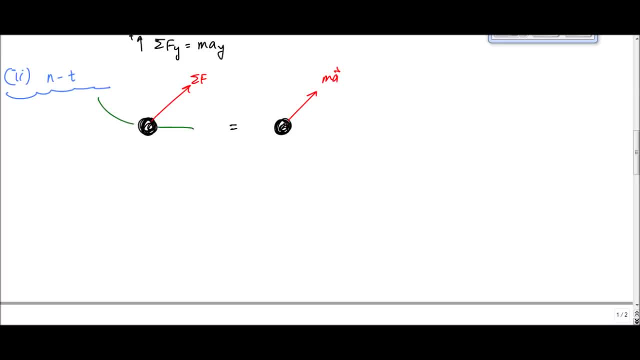 M-A. OK, Right here, And I have Again this path. it was going on some path like this right here And the N-T coordinate system is defined. Oh, anyway, whatever The N-T coordinate system was defined on the element or the particle itself here. 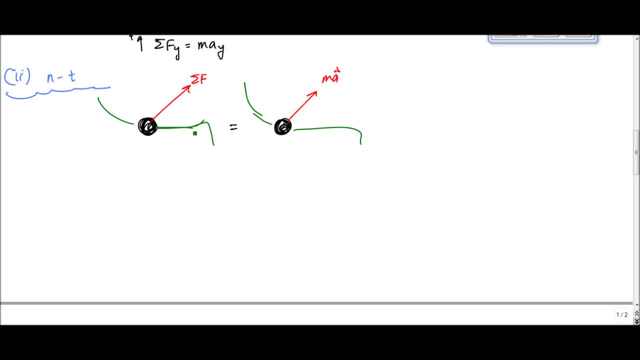 And so here the plus normal or plus tangential direction was tangent to the path. OK, plus T or in the direction of increasing path. So if this was my Velocity vector here, if my particle is moving in generally this way, or this velocity vector is tangent to the path, at that point here's my plus T and my plus N. direction was defined as towards the center of curvature of wherever that particle is plus N right here. 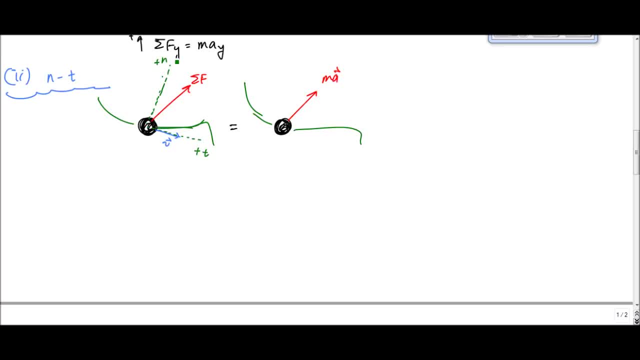 Bam, Let me give it some more plus N right here And then here I would make that same drawing over here. This would be that plus T, And this would be that same exact same plus N Right here And now. I would just break these up into appropriate components. 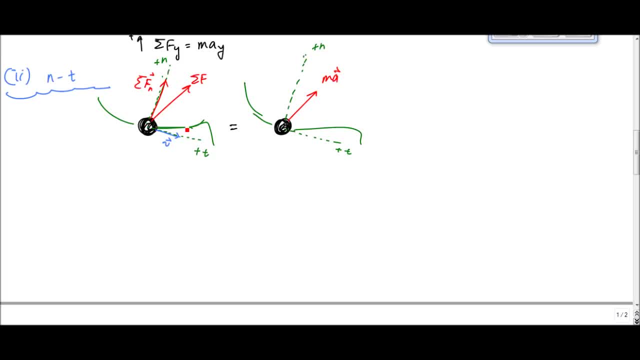 This would be some of the forces in the N direction. I'd have a sum of the forces- Oops, Let's do that a little bit more precisely. So I'd have a sum of the forces in the tangential, And here I'd have a M-A-T and an M-A-N. here. 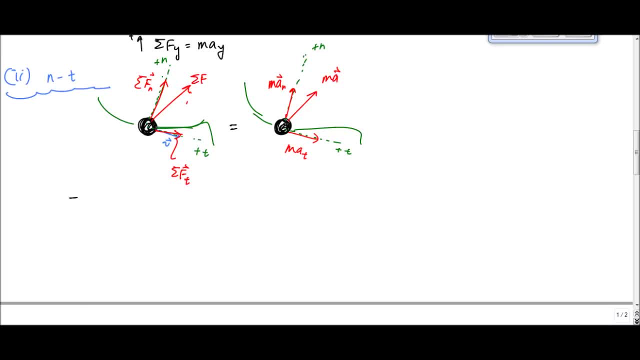 OK, And I just go through Again. summation of all the forces. Summation of all the forces in the N is equal to M-A-N. Summation of forces in the T is equal to M-A-T. right here. 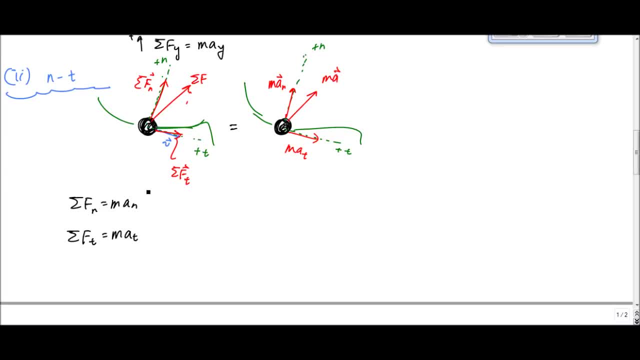 And this, if you remember what the normal acceleration was in NT components, right here, this was M V squared over rho, where rho is the radius of curvature, And then this M was D-V-D-T, And this coordinate system had the specific advantage. 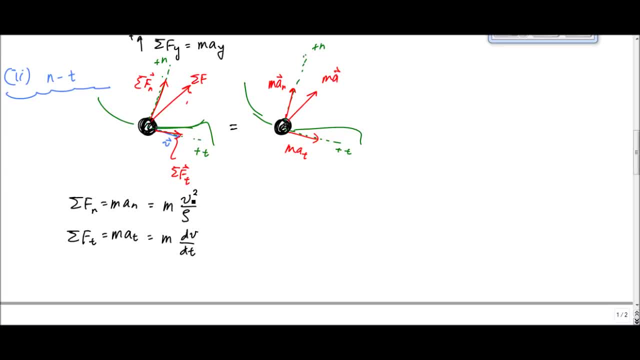 so that when you looked in the tangential direction it looked like 1D motion. The centripetal component right here, the centripetal acceleration was often. That's what this V squared over rho was sometimes called right here, But this is it. 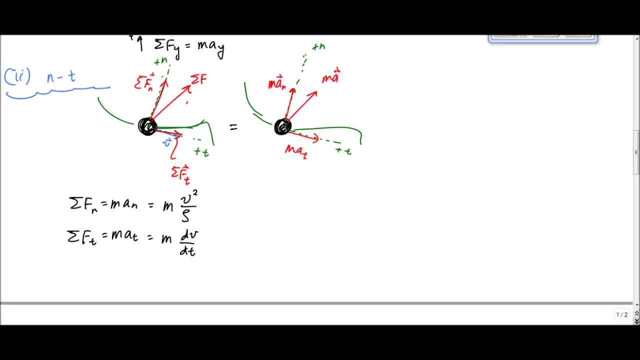 This is what you would use if you this exact same problem, exact particle in the exact same motion, but in NT components. And then, last but not least, you could attack this exact same problem in radial and transverse. Radial and transverse. 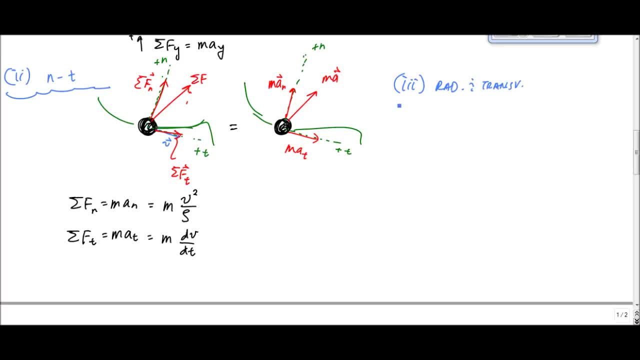 Or what sometimes people call polar coordinates in 2D right Or cylindrical in 3D, right here. But here again, if I have the exact same particles, exact same drawings, right here, this right here, my sum of the forces, bam, like this: 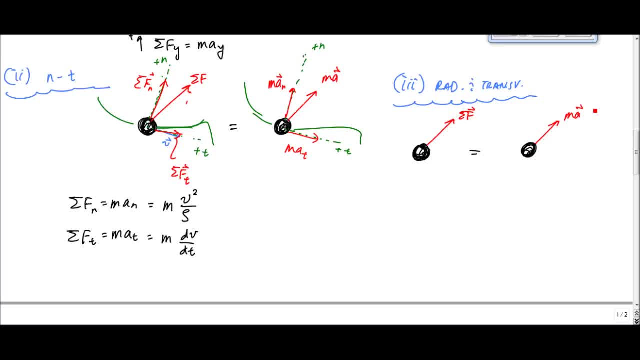 Mass, an inertial term like this, right here And now. just like the Cartesian coordinate system, the radial and transverse also needs an origin, And so here let's say here, here is this path, here That this was traveling on, right. 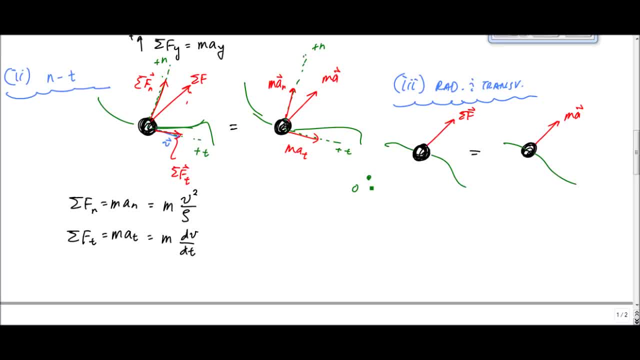 And here I have this origin here. Here's my origin of that coordinate system. My radial direction is defined as from the particle. My positive radial direction is defined as from the origin to the particle. So there's a line here. If you can envision a line going like this, 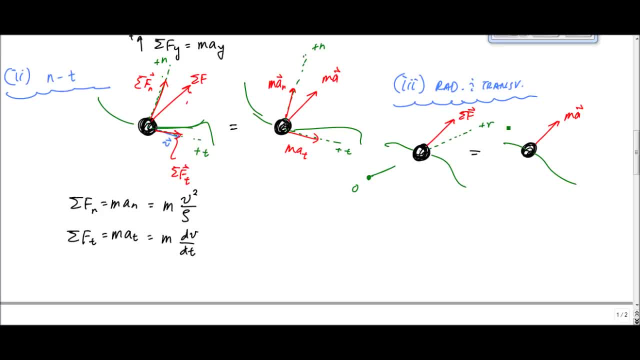 And so this is my plus r direction And my plus theta direction. okay, My plus theta direction Is 90 degrees to the r. So here in going counterclockwise, So this would be my plus theta orientation. And so same thing here you know, for this exact same particle right here. 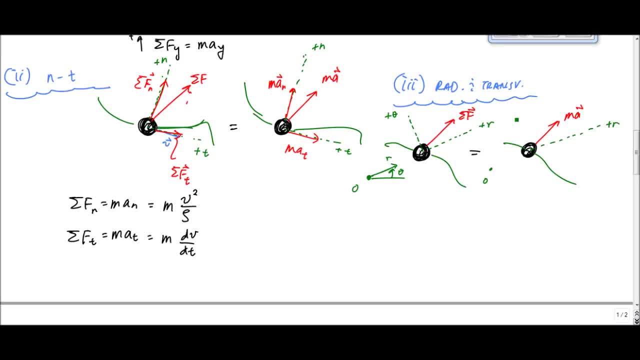 I have my established my plus r or my plus radial direction And my plus theta in the 90. And these two drawings are exactly the same, other than that this is an inertial term over here on ma And this right here is the external forces on this left side, right here. 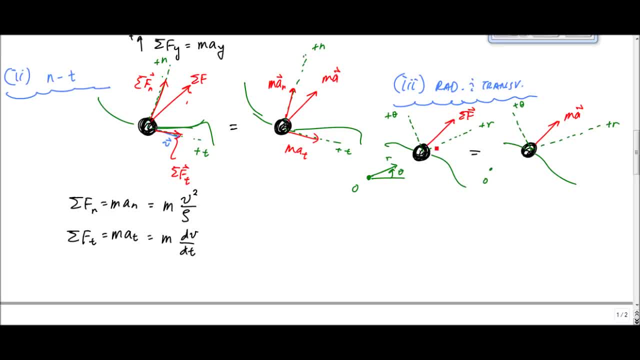 And again you just break up into components, right? So here you have this sum. you know, bam, This would be my sum of the forces in the radial direction, Sum of my forces in the transverse right here, And then same thing here. 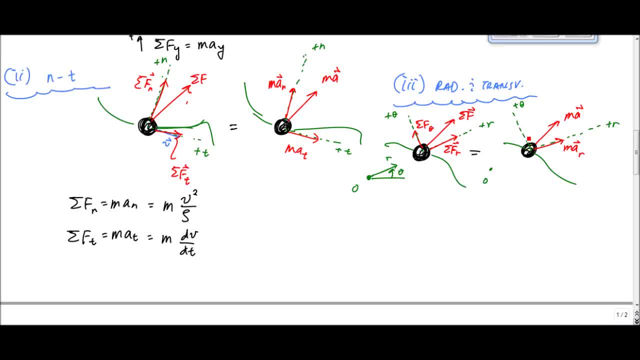 My inertial term in the radial direction And my inertial term in the transverse direction right here. And then I go ahead and I apply the equation Newton's second law, or the equation of motion in each direction. Sum of the forces in the r is equal to mar.